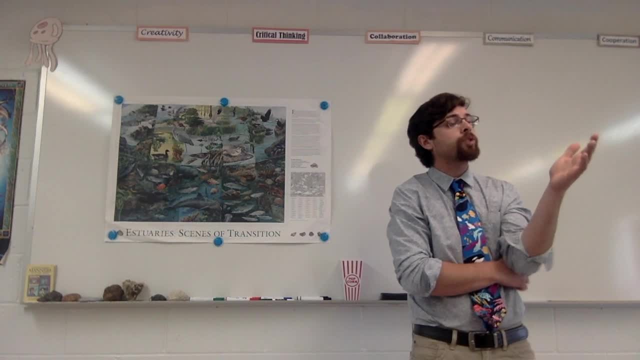 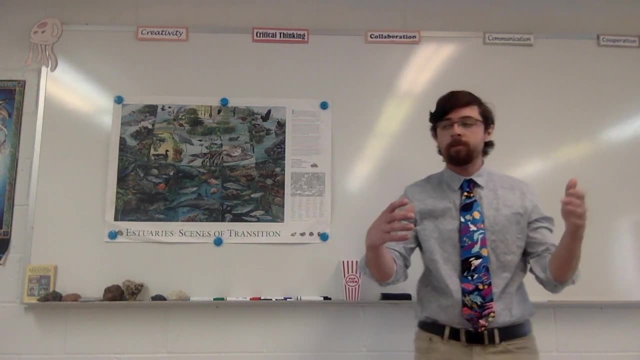 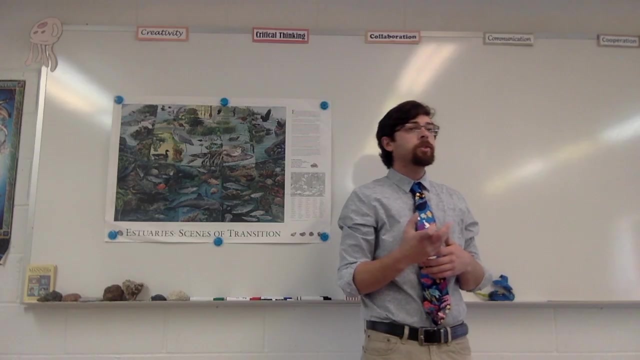 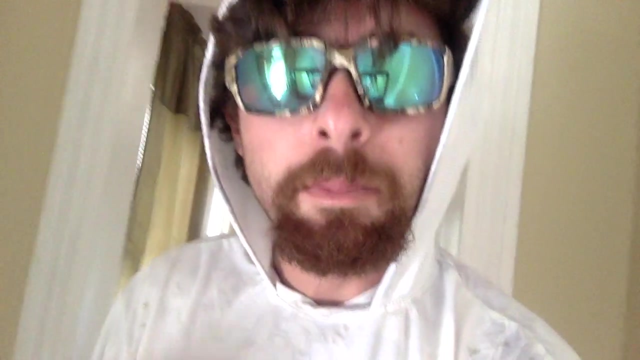 important to note that estuaries right are transitions from from terrestrial, from land habitats to marine habitats. right, and so there are going to be lots of zones of transition or lots of scenes of transition. right and so why class? are our estuaries important? bees and birds and plants, protozoans, Blake, how do you? 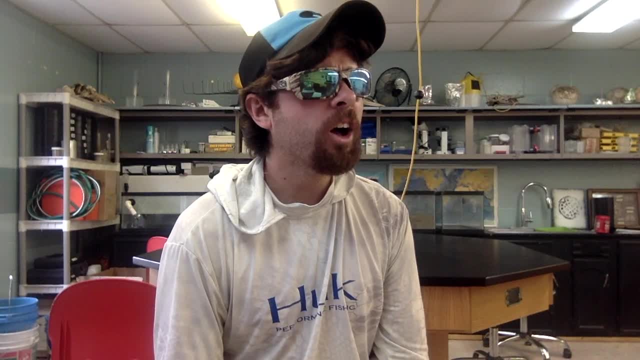 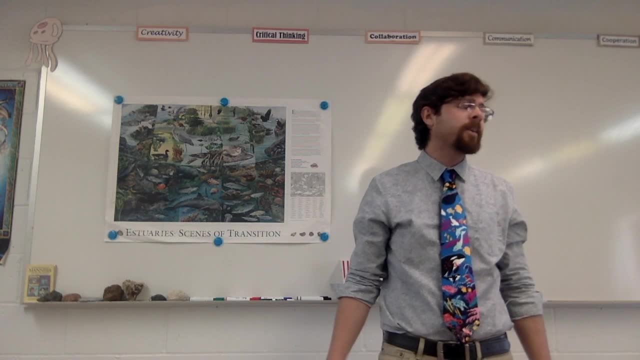 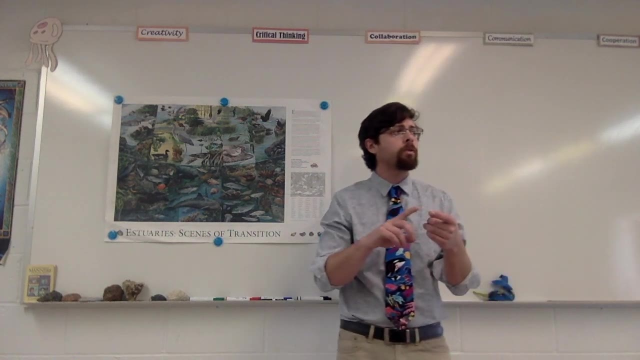 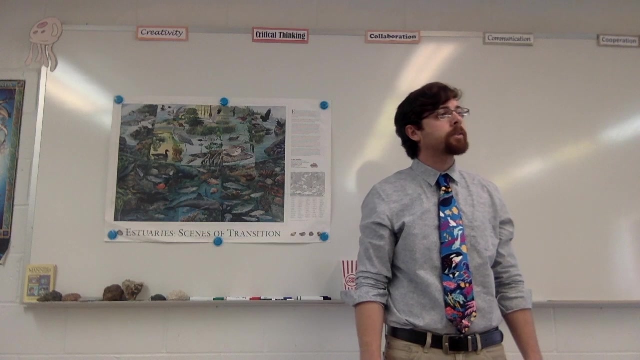 know about protozoans. huh, oh, saw it on a Nat Geo documentary, bro. well, yeah, yeah, okay, well, I guess you're right. but why okay? why is the species richness and the overall biological diversity and abundance? why are they so much greater in estuaries compared to other habitats? well, according to my calculations, let me 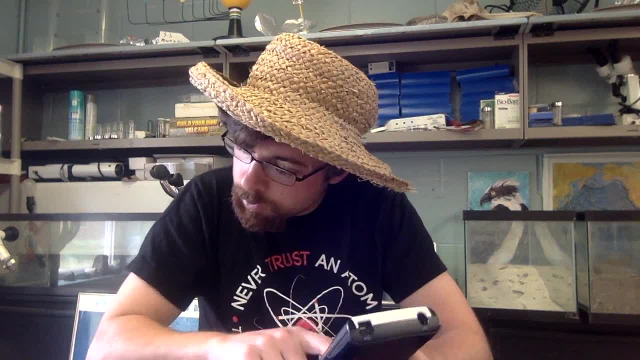 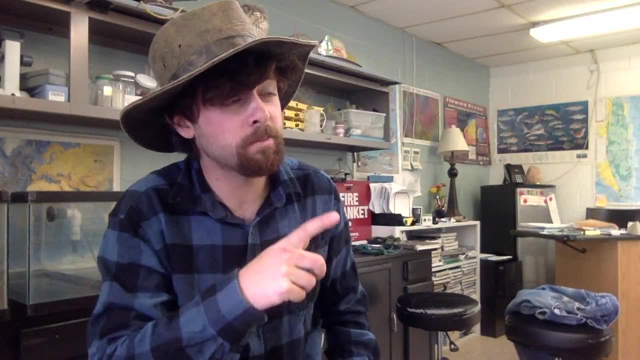 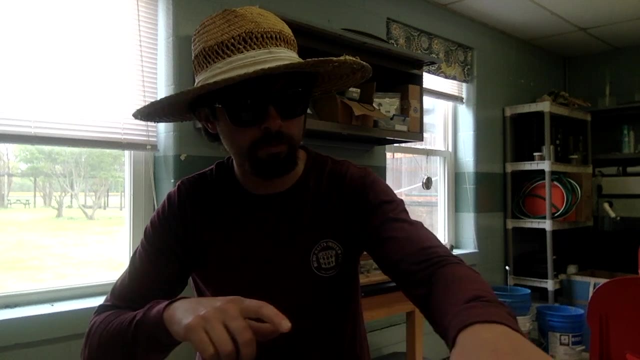 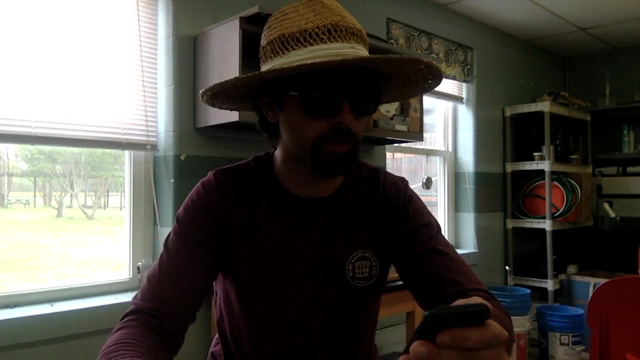 do a quick. the Nature Conservancy at Brownsville is very close to the mainland and, depending on the watershed size, lots of nutrients could wash into the system. hold on bros keys, use my app, calculate the size of the watershed, how much rainfall receives. well, that's impressive. get back to me on that. 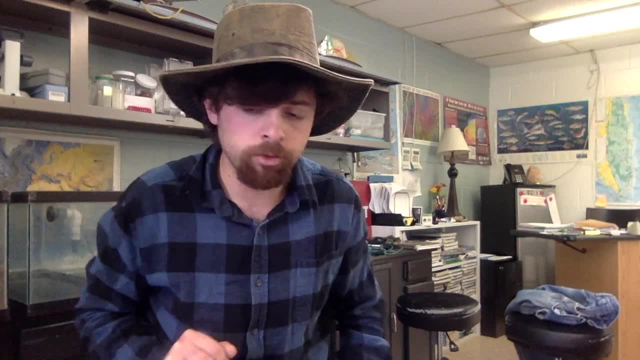 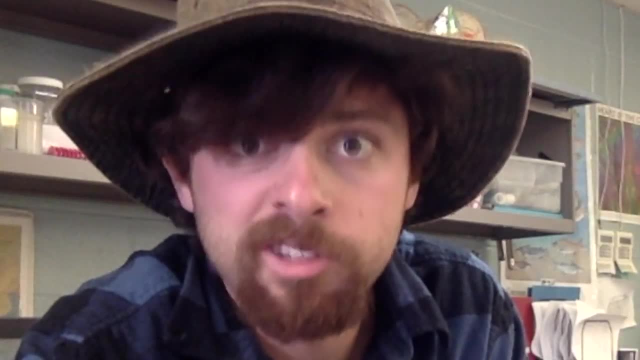 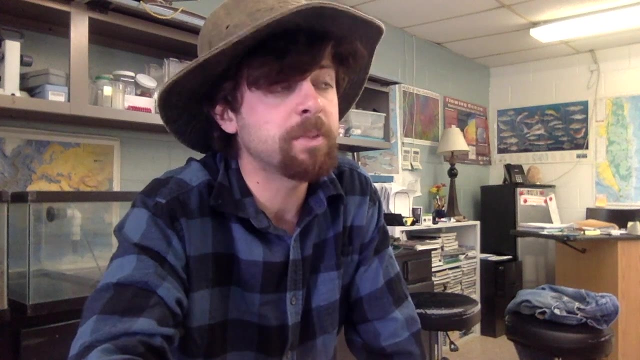 well, that's impressive, get back to me on that. well, that's impressive, get back to me on that. look, mr Carlson, the real reason why there's so much diversity is because there are small changes in the topography and the bathymetry. all right. these changes create small micro habitats that only certain species can. 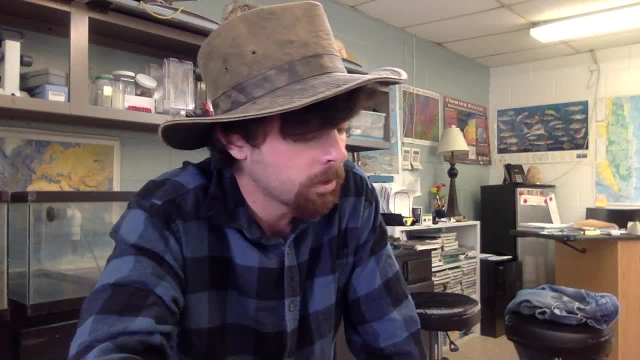 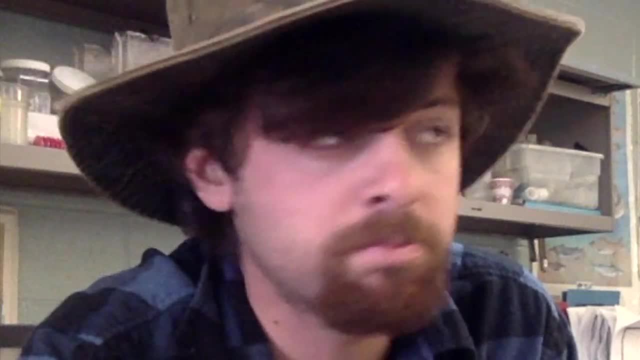 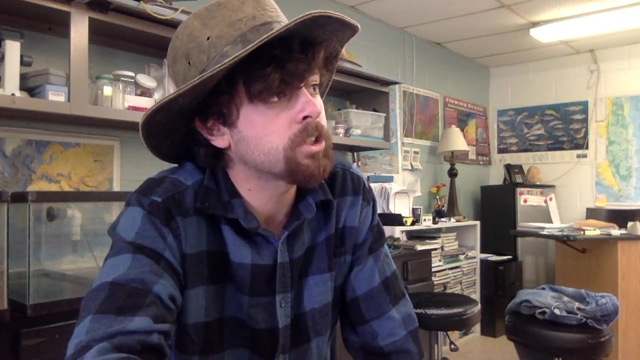 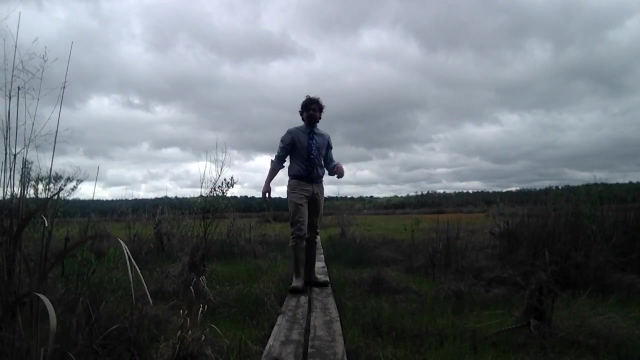 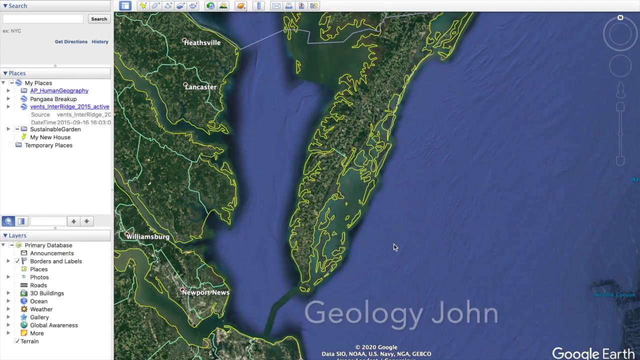 occupy species tend to favor environmental conditions and thrive best in those habitats. things like competition, predation, behavior, life larva disperser or tolerance of organisms they control these locations nailed it all right. welcome to Brownsville. so I want you guys to go out and record something that you find interesting. John, here I decided to stay. 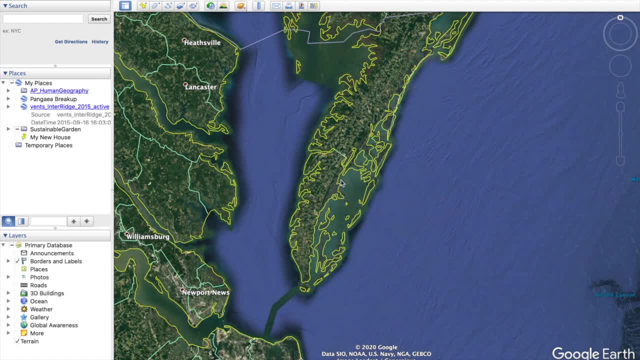 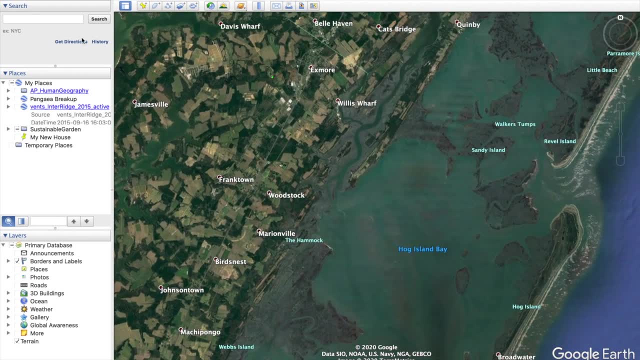 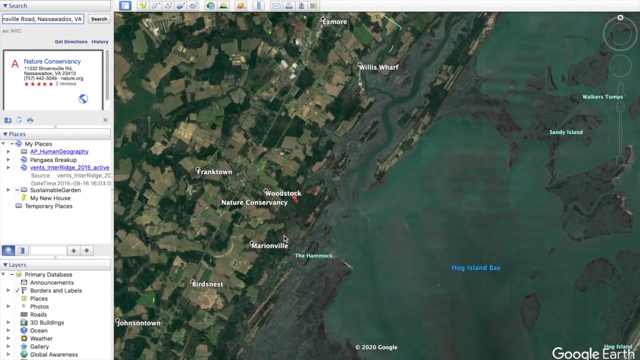 in the car for the time being. take a look at the landscape from the aerial. my geologic perspective requires me to take a look in the air first. take a look at some things. so let's type in: yes, this is where we'd like to go, all right, take me there, Google, but we are actually. 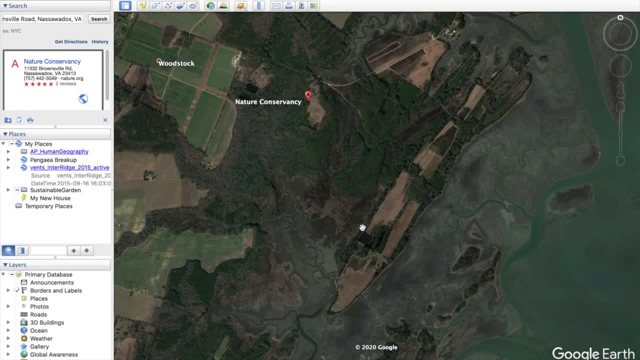 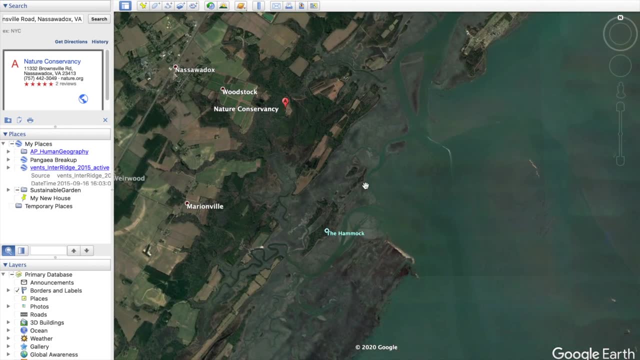 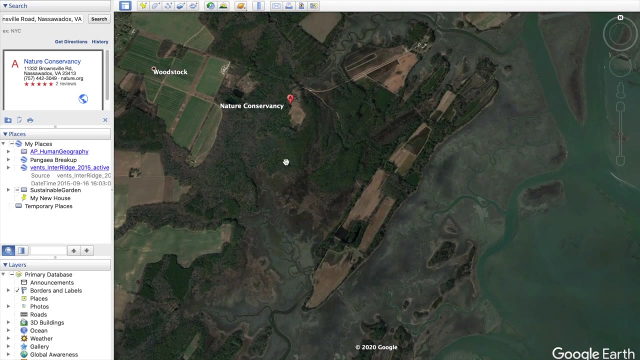 going to be taking this path right here down to this wetlands. some tidal influence. it looks like a little peninsula right here here's a big lagoon, okay, so that's the situation. I'd also like to check out some soils. I love me some soils. what type of soil do 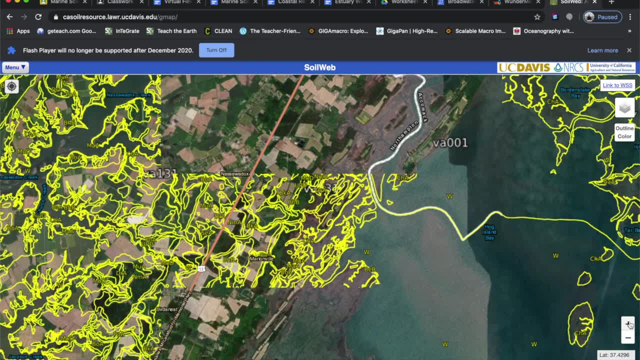 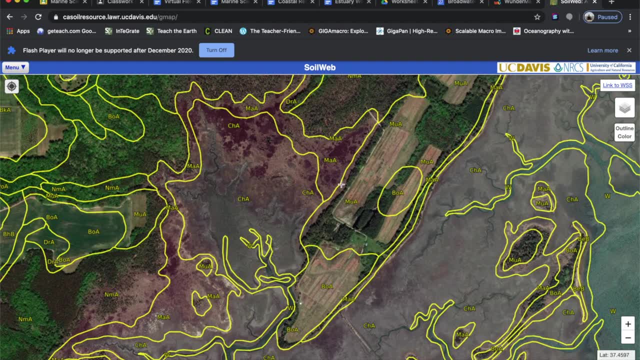 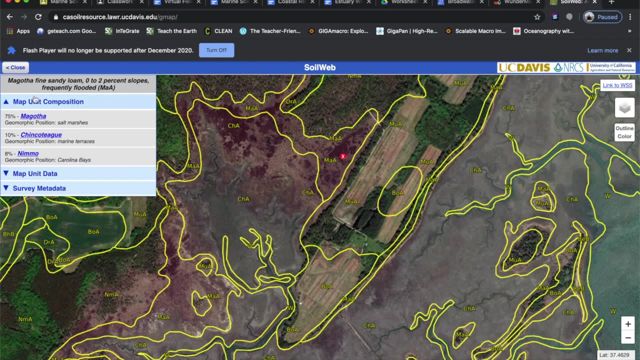 we want. oh bloody, look at all the different types of soils. let's zoom right on in here. okay? so here's our wetlands, right? so let's take a look at what type of soil is right here. I'm on soil web at this location. we've got 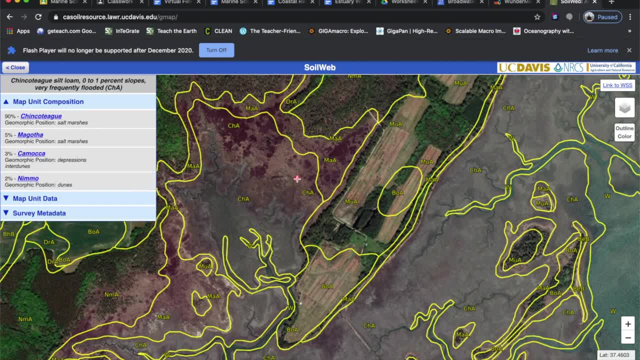 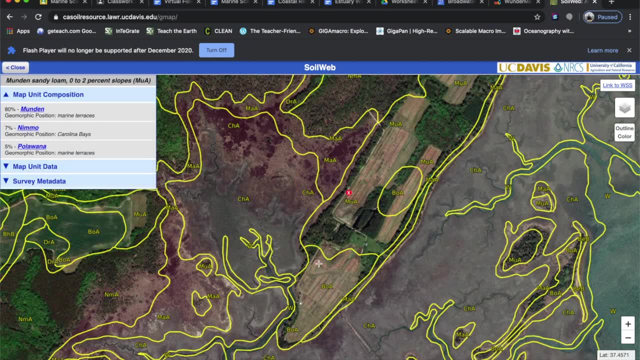 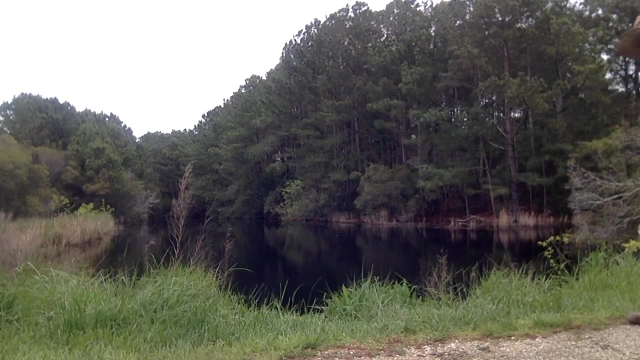 Magotha- fine sandy loam. we've also got some shingatig silt loam, got some Bunn sandy loam and some Bojack fine sandy loam. so let's go take a look. if we can find those in the field, let's get it. 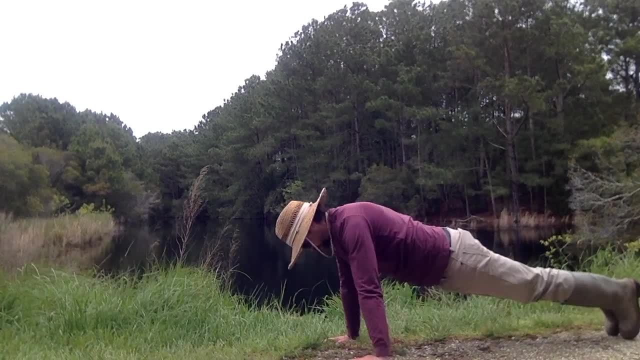 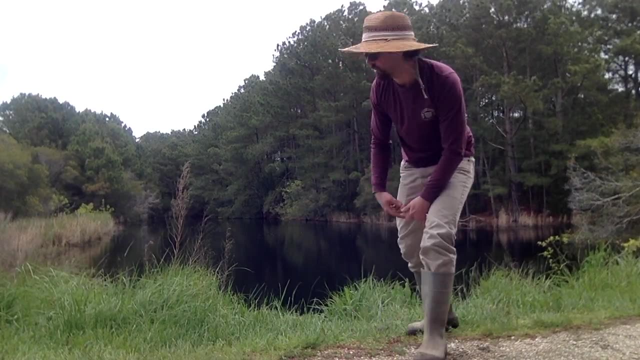 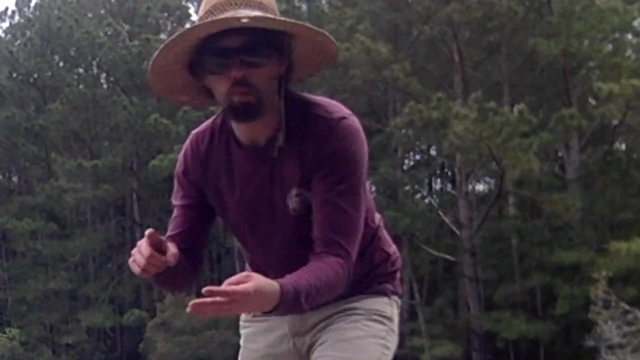 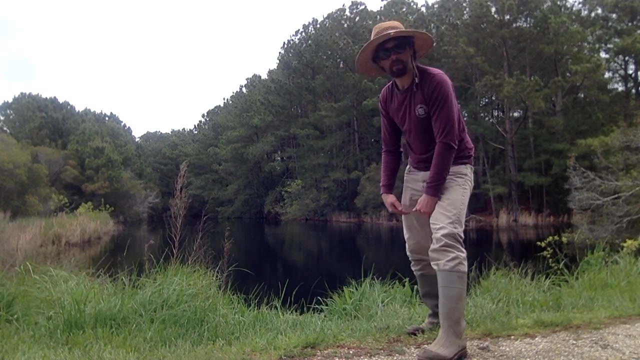 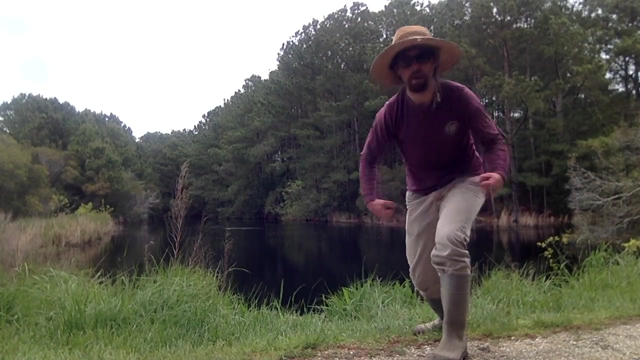 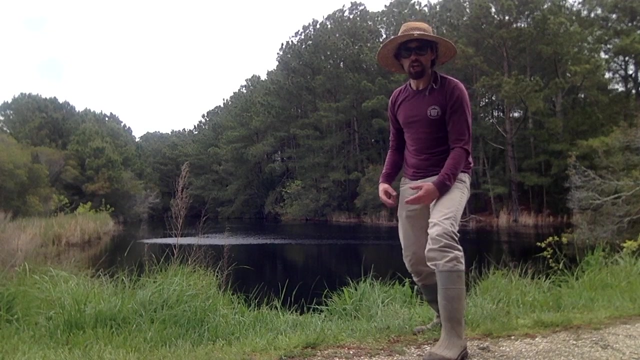 one, two, three. it's your boy, Philip, here. talk about the physics of this tidal creep. the variables of temperature, salinity, wave action, wave dull, they all effect the organisms right here because the system is flushed twice daily in a semi diurnal pattern that exposes them to different levels of temperature, salinity and even desiccation. 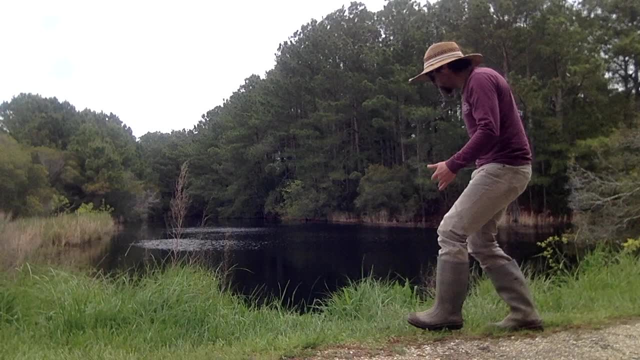 so, based on all those parameters, you're only going to find certain organisms in soil that are in this tubal system, that expose them to different levels of temperature, salinity and even desiccation. so, based on all those parameters, you're only gonna find certain organisms in soil that are in this tubal system. 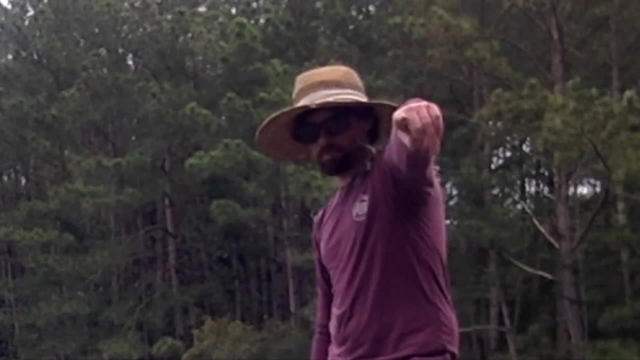 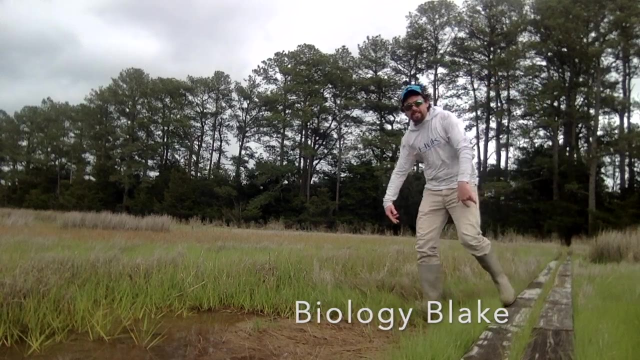 in certain spots. Let's go. Would you check this out? I've got some mud. What it do? bros and broskies? I'm out here in this swamp- You want to call it a swamp- Chilling with some marsh grass yo.